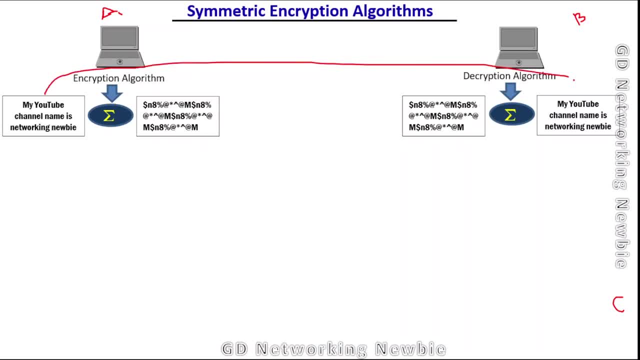 original message. like you can see here, after decryption the user has got the actual message which was sent. so now this: in this encryption and decryption scenario, the problem is that that if there is any third user with the right decryption algorithm and somehow if that third user lets user see if that user is able to receive that, because this will be kind of wireless channel. 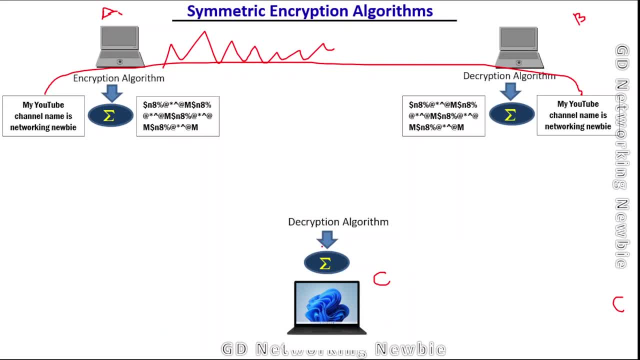 in between them. so it means the third user can also receive that message. and if, for example, it is not wireless, let's say this is wire, simply wire, so they can do wire. maybe they can also receive the decrypted message and with the right decryption algorithm they can also receive, or they can also recover, that same message. 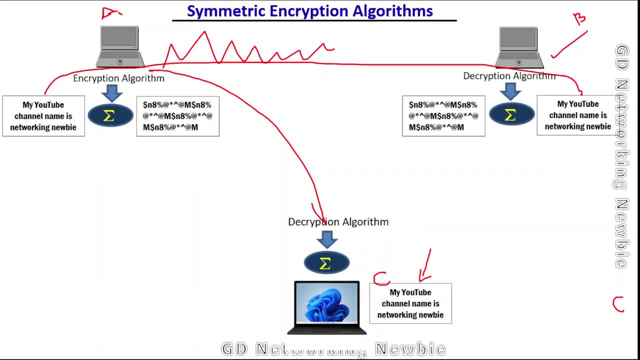 which actual destination was able to recover. so it means there is some problem in this case. now, to avoid this problem in symmetric encryption, both the sender and receiver- they use a common secret key, a key which is known to each other and only they know about that secret key. so they use. 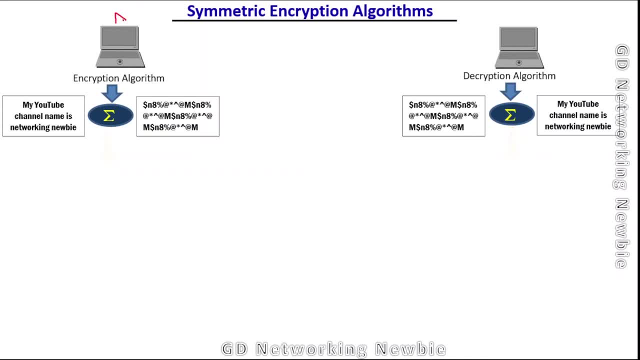 that particular secret key which only belong to user A and user B and no one else knows about that key. so they use that key in addition to the actual encryption algorithm to encrypt the message and at the destination, the destination B also uses the same key to decrypt the message. 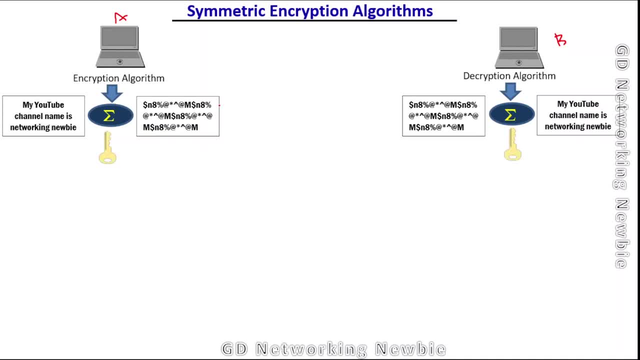 now, in this case, even if there is any third user, if that third user is going to receive this message and you're going to use this, let's say you're going to use this decryption algorithm. so decryption algorithm are actually made public. everyone knows about decryption algorithm. 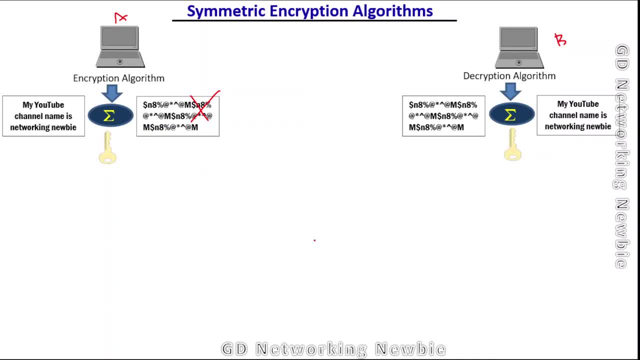 so if they receive it and they use this, the common known decryption algorithm, to decrypt the message, then they will not be able to decrypt the message, because for decryption they also need to have this key and no one else has that key. so that is the message, and in this case now the message is that the symmetric cryptographic